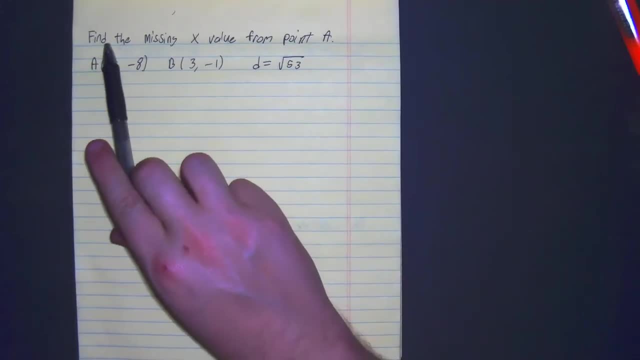 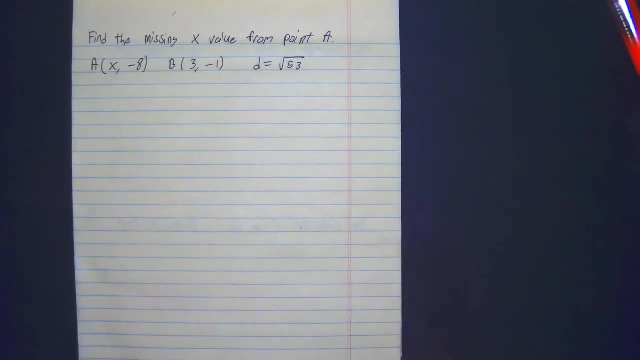 All right. so this says: find the missing x value from point A. So we're giving two points and it's distance. So we're using the distance formula but we're missing a point. So we need to figure out what is that exact point? So what is that x value to make this whole statement true? 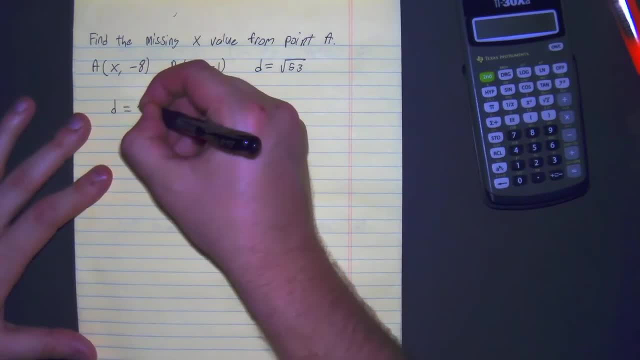 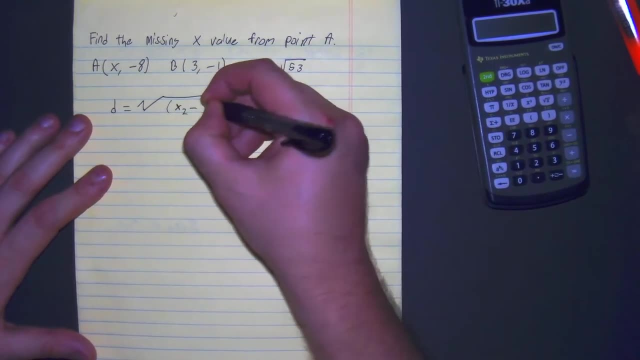 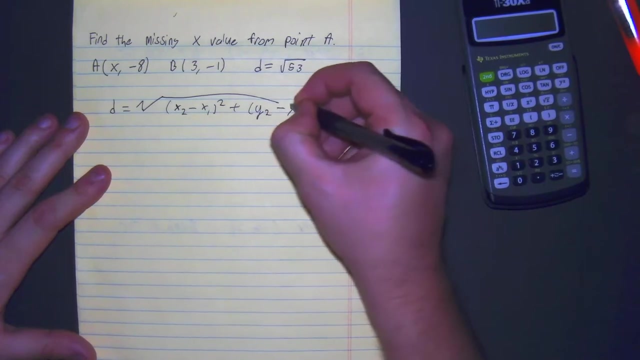 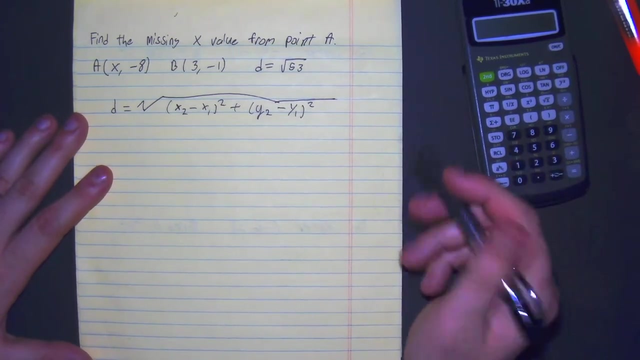 Distance is equal to: oh, that's a horrible radical. Oh, that's fine. x2 sub 2 minus x sub 1 squared, plus y2 minus y sub 1 squared. Just pretend that's not curved. Now we know we need to label it x1, y1, x2.. 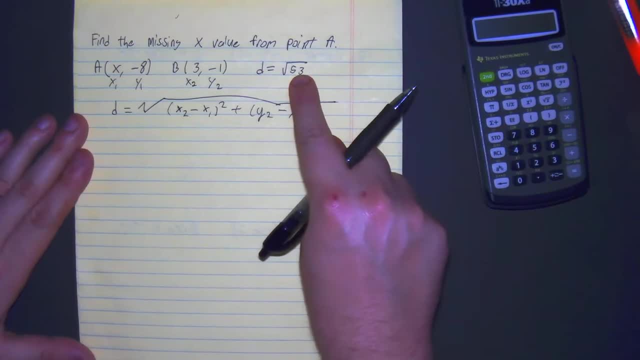 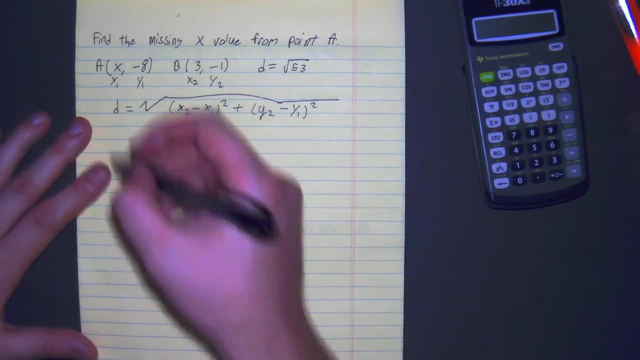 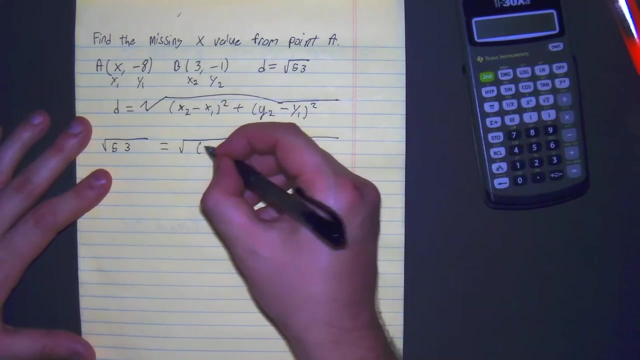 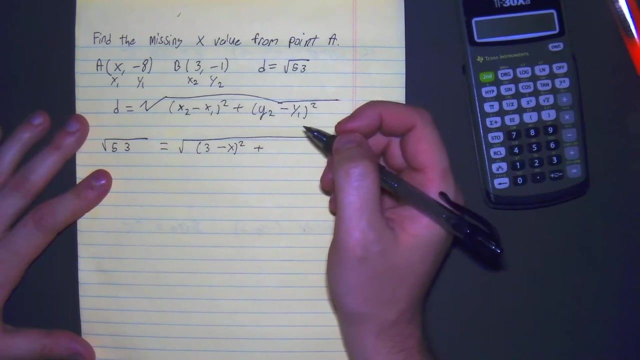 x2,, y2, and that's our distance. So I'm going to plug all this stuff into this equation. We're going to go from there. This is a little bit more advanced than what we've been doing. So we have square root. 53 is equal to the square root of 3 minus x, squared plus negative, 1 plus 8.. 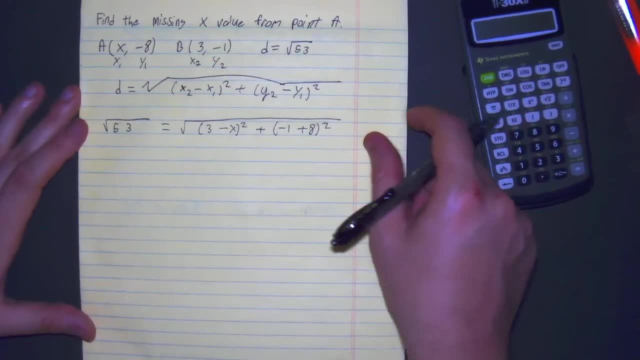 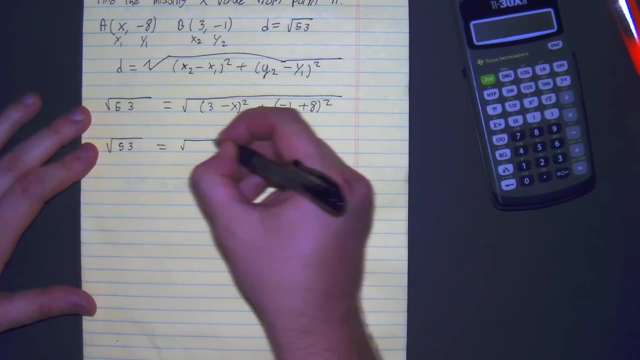 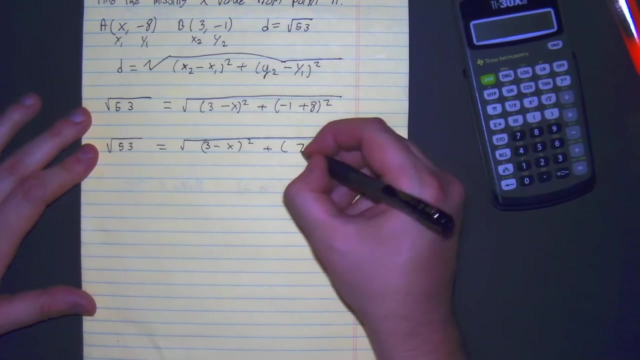 Square root of 3 minus x, squared plus 7 squared. The first thing you need to do is you. we need to get rid of this radical, So let me rewrite it: Square root 53 is equal to the square root of 3 minus x, squared plus 7 squared. 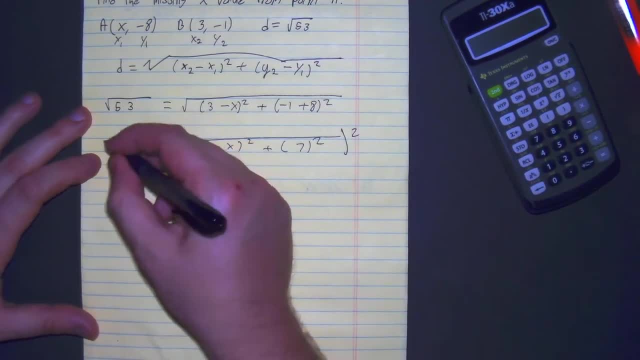 First thing you need to do is we need to get rid of the radical. So we square both sides. That means the radical cancels and the square root, or the radical cancels all right. So we get a square root and a radical. 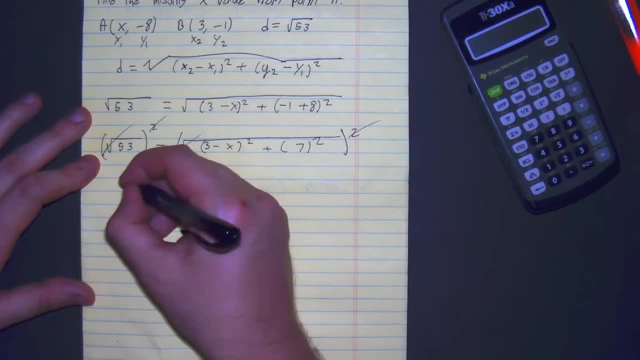 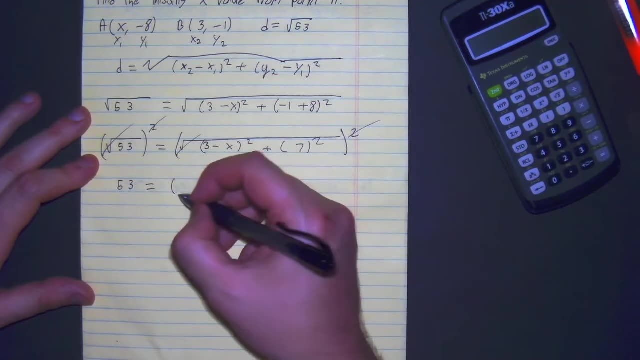 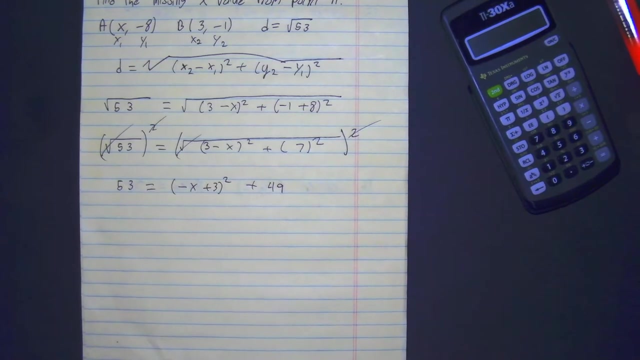 That's the first thing you need to do. square cancels, this cancels, this cancels. so now we're left with: 53 is equal to negative x plus 3, squared plus 49.. So what's going to happen with this is we need to double it. it's not going to become. 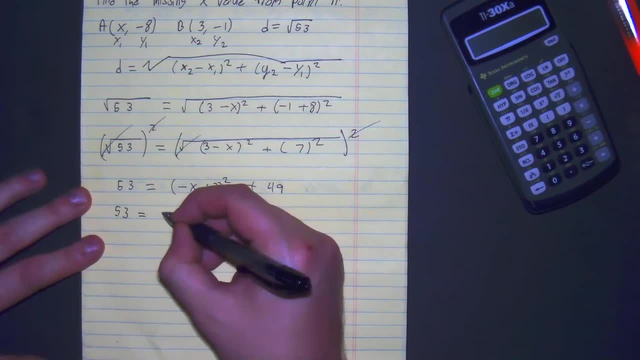 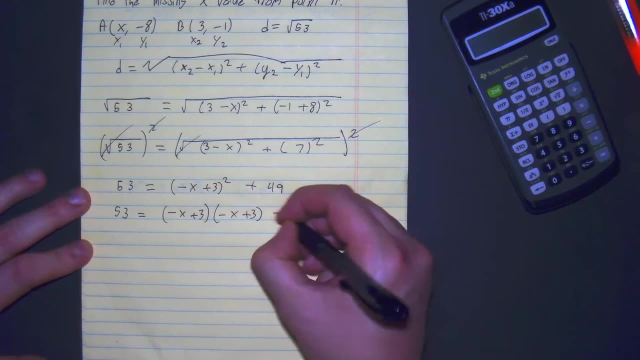 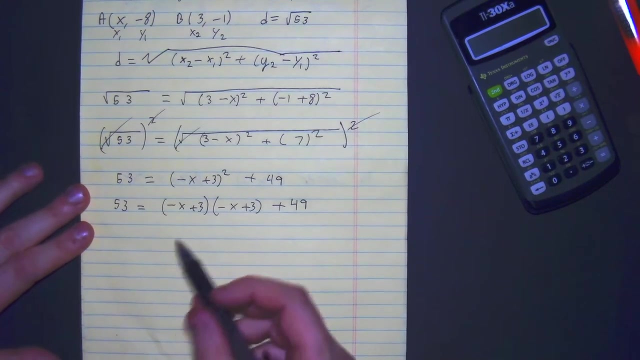 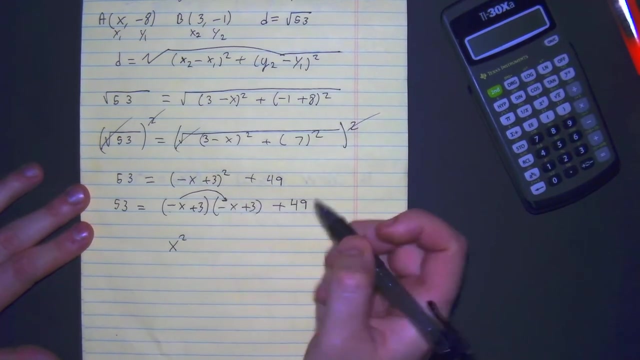 what you think it is. So now we have: 53 is equal to negative x plus 3 times negative. x plus 3 plus 49.. From here you need to distribute, So x times x becomes a positive x squared. so we have x squared. 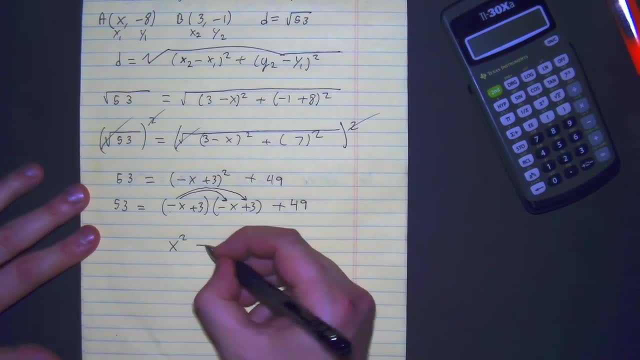 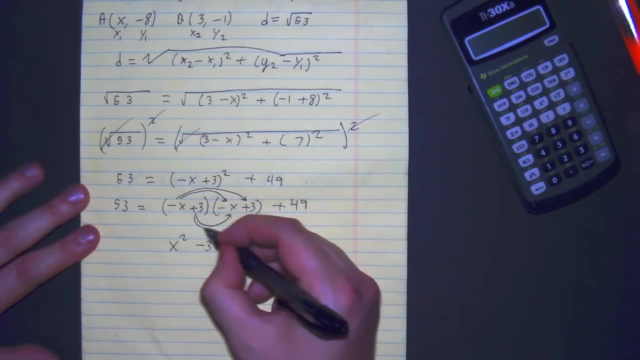 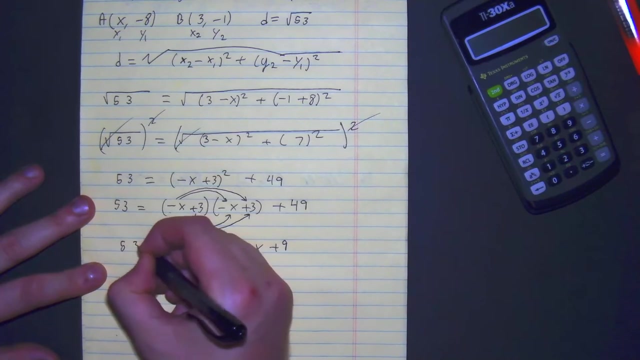 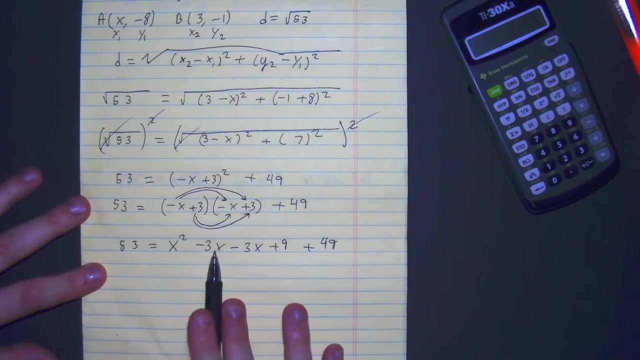 Then we do negative x plus 3,, which will become minus 3x, And negative 3, or 3 times negative x becomes minus 3x, And the last one is: 3 times 3 is 9.. So we're left with this: 53 is equal to x squared minus 3x, minus 3x plus 9 plus 49.. 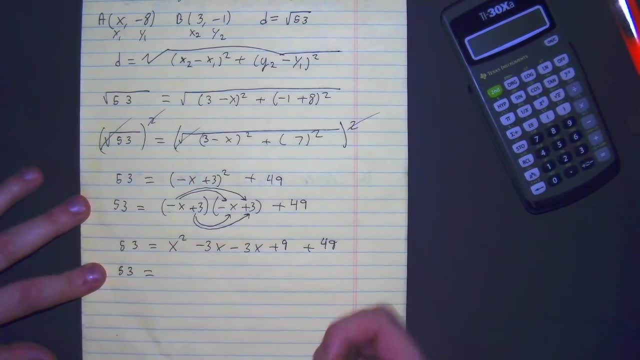 So now we need to start simplifying. 53 is equal to x squared negative, or minus 3 minus 3 minus 3.. Negative: 6x 9 plus 49, 58, from here I need to subtract this over, because we do have to. 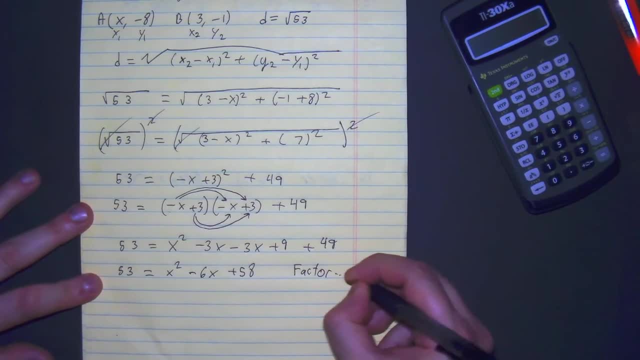 factor equal to 0, with the factor, so we have to equal to 0.. So minus 53, minus 53, 0 is equal to x. squared minus 6x, 58 minus 5 will be 5.. So how do you factor? 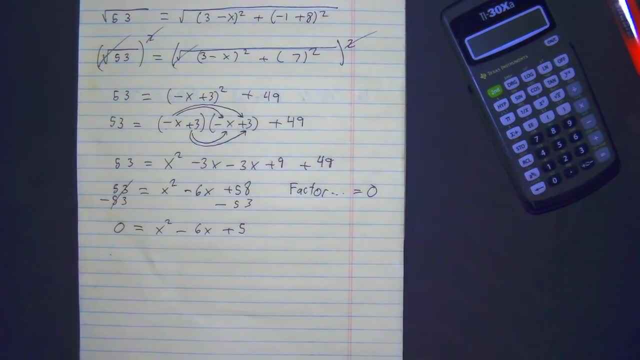 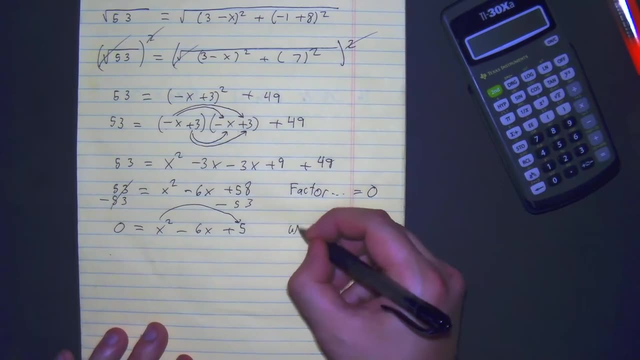 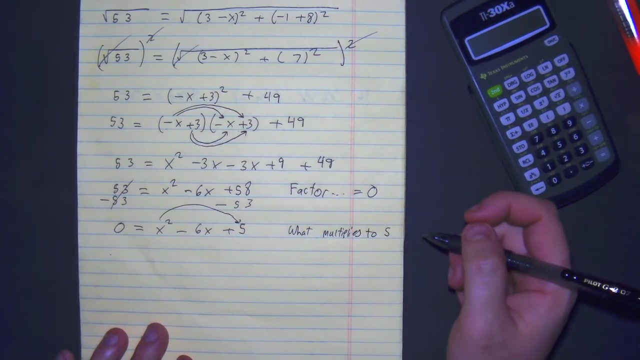 Well, this is back to your Algebra 1 course. So how do you factor? So 1 times 5, this gives us what. Multiplies 2, 5. But adds 1. So 1 times 5, this gives us what. Multiplies 2, 5. But adds 1. So 1 times 5,. this gives us what Multiplies 2, 5. But adds 1. So 1 times 5,. this gives us what 2.. 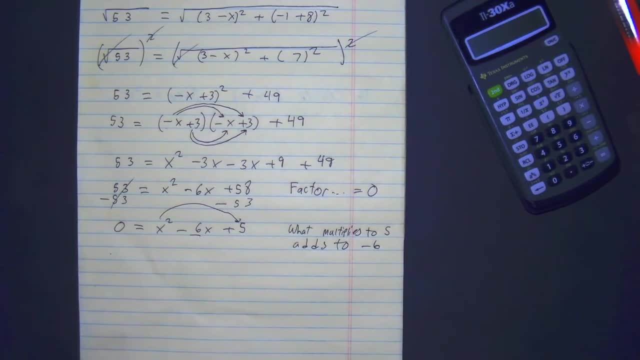 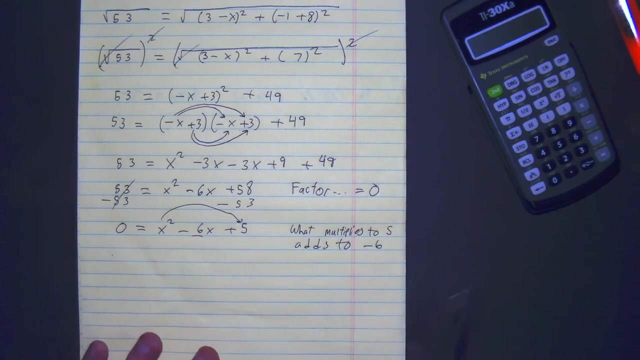 Negative 6.. So it multiplies the 5 but adds the negative 6.. Alright, so the way you're going to figure that out is you need to start making the table. Well, let's try the easiest one: 1 and 5..